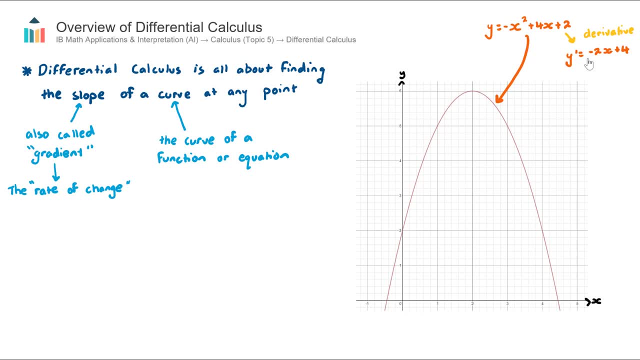 that detail. before we start finding equations of tangents and normals, before we start finding turning points and then understanding what they mean in the context of optimization, I think it's important to start by actually sort of visually understanding what are we doing here when we differentiate? 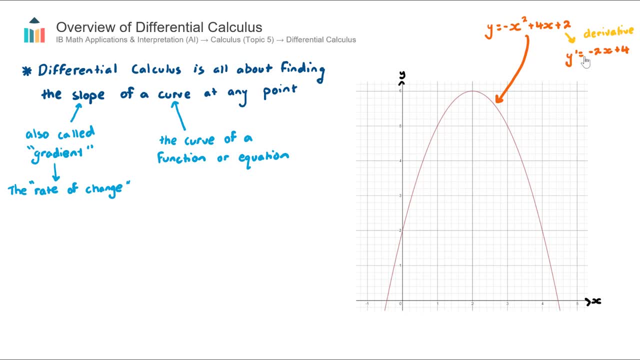 What are we doing here when we differentiate an equation and we substitute in an x value? So that's, I think, where I think it's a good place to start here in this subtopic of differential calculus. That way in future, when you get an equation and you find the derivative, you 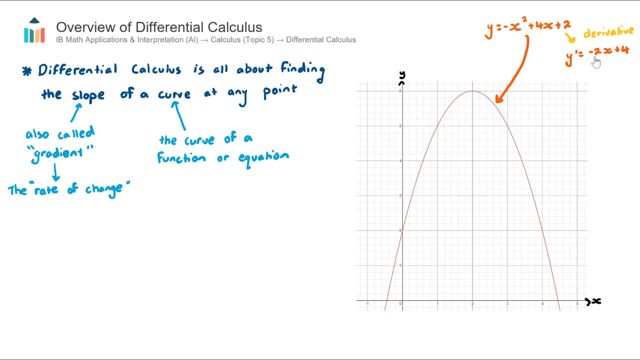 actually know what it kind of means in the context of the question. Okay, so let's start by looking at this curve here. This is the curve of this equation here. this is a quadratic: negative x squared plus 4x plus 2.. It's a quadratic, it has a turning. 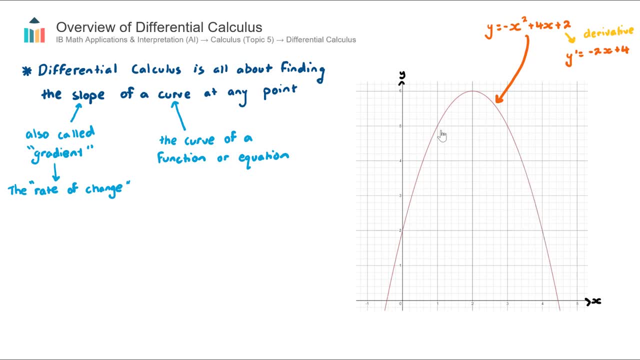 point here and then it goes back down- And I want to narrow in on this particular coordinate here, And we can just read off the graph here that it has a x value of 1, so this point here has an x value of 1 and it has a corresponding y value of 5.. So this has a y value of 5.. So this coordinate. 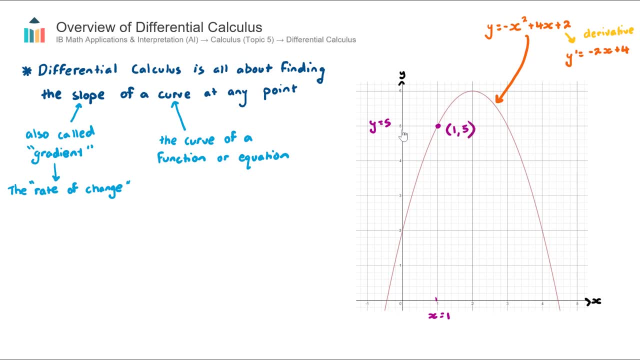 here is 1 comma 5.. And also just to be clear what this means is, if I was to substitute in x equals 1 into this equation, the left hand side would equal 5.. So the corresponding y value at an x value of 1 is equal to 5.. 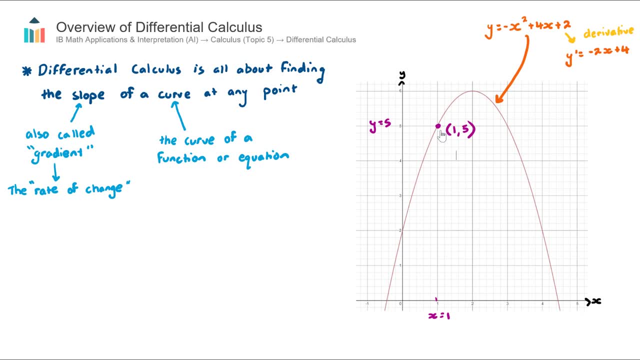 Now, at this point, what if I was to ask you the question: what is the slope of this curve? at this point- And this is what differential calculus is all about. And you say, okay, well, it looks like it's sloping upwards, but how do I actually find out what that slope is? And if I was to visualize, 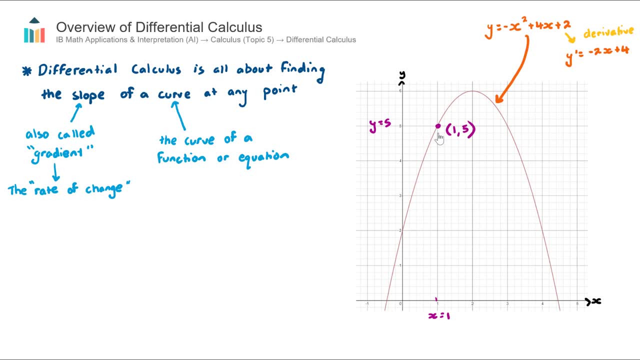 the slope. the way that we visualize the slope at this point is to actually draw a straight line that runs parallel to the curve at that point, A straight line that looks something like this: Now, there's actually a proper word for this line, and this word here is a tangent, So let's write. 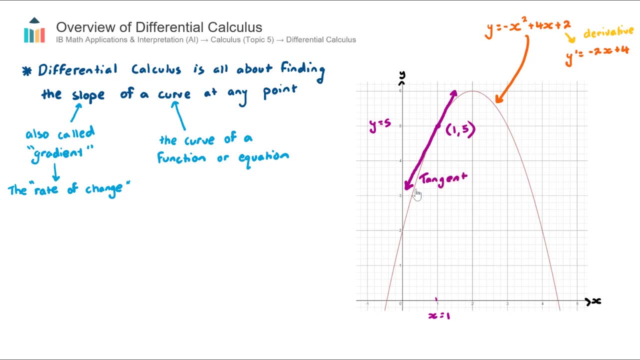 that in. So this purple line here is actually the tangent to the curve. at x equals 1. And this actually gives us the slope of the curve at this point. And we would find that by actually finding the gradient of the tangent Now recall that straight lines. 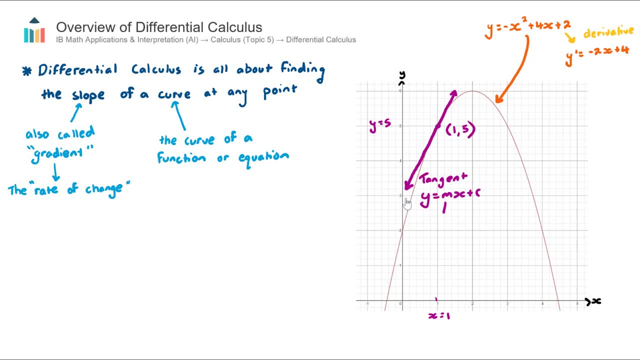 have the equation: y equals mx plus c. so this m value gives us the gradient of this purple line, which happens to be the slope of the curve, at x equals 1.. Now that is what differential calculus is all about. Differential calculus is is all about finding the slope of a curve. 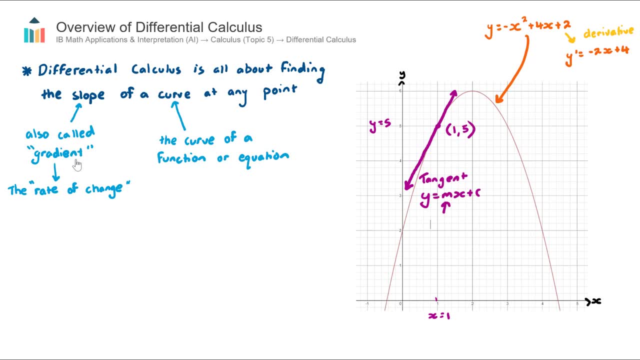 at any point, and we all, and we also call the slope the gradient, and that comes into the topic of rate of change, which, in other words, how much is this curve changing at x equals 1. Xs are giving echelonedy terms, So let's bring that up. So let's. 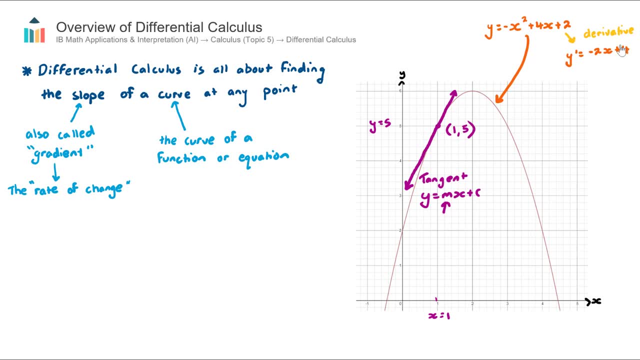 go ahead now and actually find the gradient of this tangent, and I already have the derivative here. the next video is all about: well, how do I get this derivative? we call that derivative y dash, or, if we're using function notations, it'll actually be f dash of x rather than just f of x. 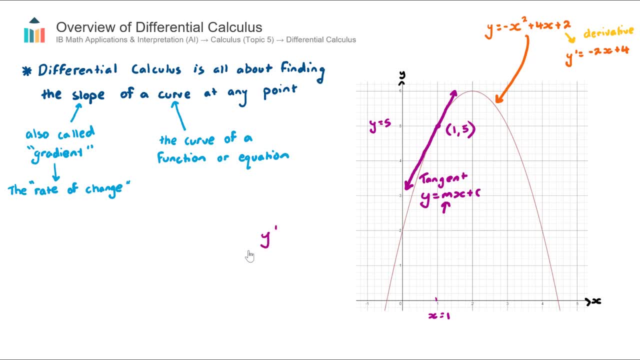 so let's just write this down here: if I have the derivative, y dash is equal to negative 2x plus 4, then at x is equal to 1. this particular coordinate here that we're interested in, y dash, will equal negative 2 multiplied by 1 plus 4. so I'm just substituting in: x is equal to 1. 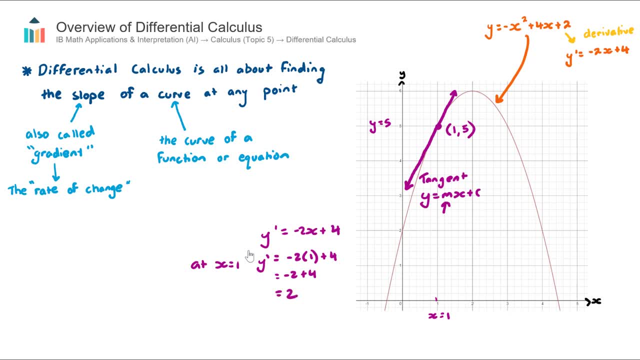 that is negative 2 plus 4 and that is equal to 2. so what that means is this purple line here has a gradient of 2 and that that looks correct. it has a positive gradient. it is sloping. it is it is going upwards, sloping from low left to high right, and this relies on some strong understanding. 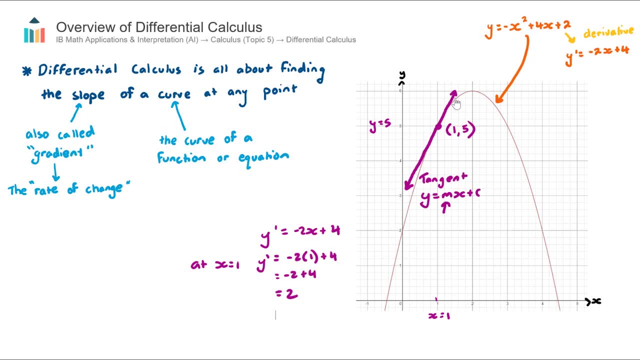 of of linear lines, straight lines. y equals mx plus c, and whether we have positive or negative gradients or negative gradients. so this particular line here has a m value, a gradient of 2. so that is what differential calculus is all about at any particular point on the curve. 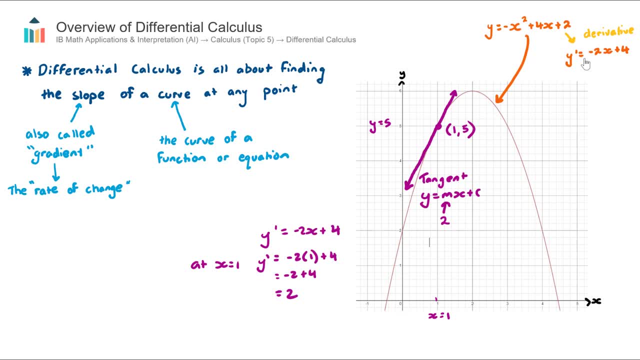 we can use the derivative to find the slope of the curve, which I think probably a better way to think about it is: what is the gradient of the tangent if I was to draw a tangent at that point? so I'll just do another example. let's look at the turning point here. 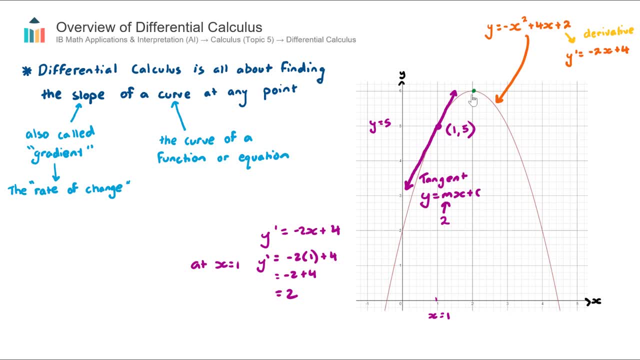 these are the two points that we're going to draw a tangent at that point. these are always interesting cases and I do have a dedicated video on turning points. the slope of the curve is actually going to be a horizontal line here. my tangent is going to be: